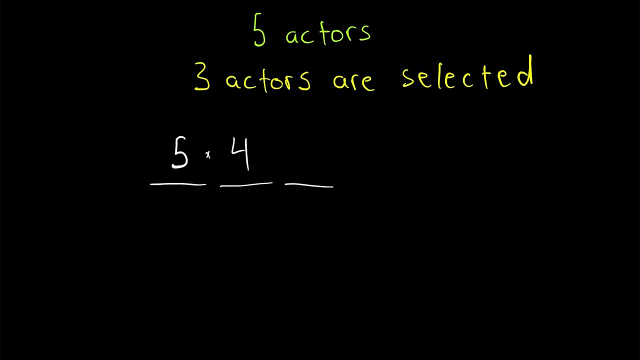 be selected first, there are four actors that could be selected second, And for all of those 20 possibilities of actors that could be selected first, then second, there are three actors remaining that could be selected third. So that's a start, but that's not exactly what we want, This number. 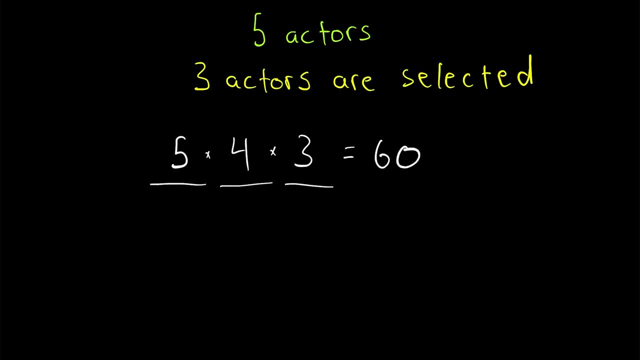 happens to be 20 times three, which is 60. That's the number of ways that we could arrange three actors from a collection of five actors. But when I say arrange, I mean order. There is ordering in this count, and we don't care about the order. So then we want to know how many. 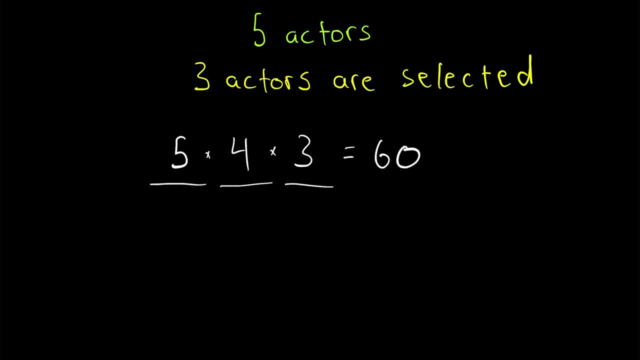 orderings are being counted because we want to get rid of the alternate orderings. Well, for any combination- that's what we do- care about the number of combinations. For any combination of three actors, let's just call them Bill James and let's say Chad- Bill James and Chad. For. 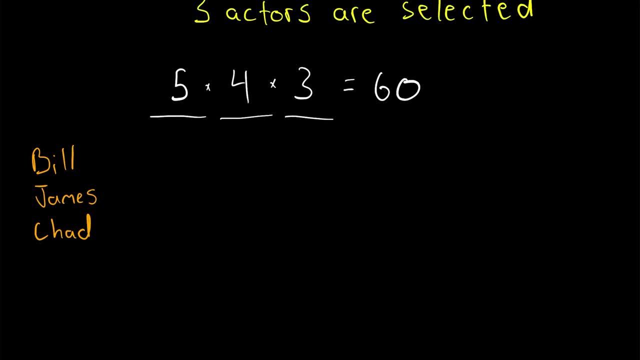 any combination of three actors like Bill James and Chad. we want to count it just once, But all of the alternate orderings are also being counted in this number: 60.. How many alternate orderings are there of three actors? Well, that would just be three factorial. That's the number of ways we 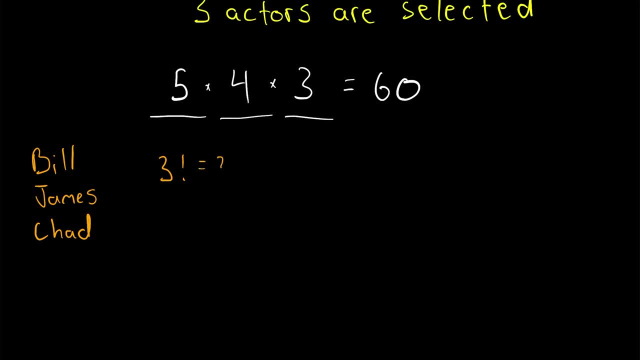 can arrange three objects in order. Three factorial, of course, is the number of objects that are being counted in order. Three factorial, of course, is equal to three times two times one, which is six. We could have Bill, James, Chad, Bill, Chad, James or James, Bill, Chad or James. 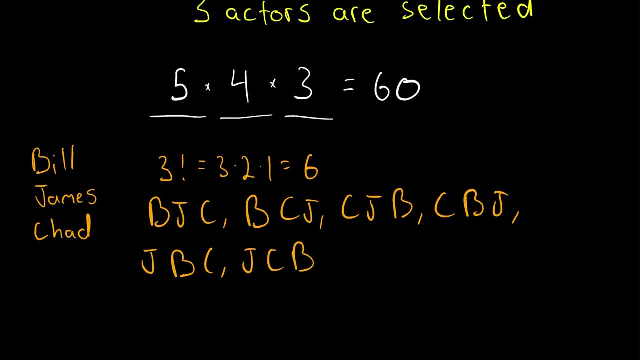 Chad Bill. Those are our six possibilities. So what's actually happening is that every combination of three actors that we care about is actually getting counted three factorial times instead of just once, which is what we want. So to correct our count: 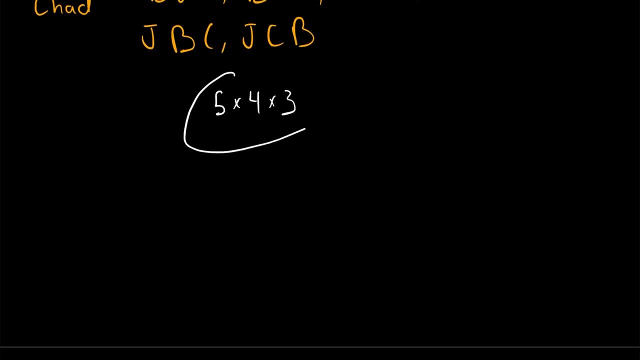 we have five times four times three, the number of ways of ordering three actors from our collection of five. But then, since every combination we care about is being counted three factorial times, because that's the number of ways of ordering any selection of three actors, we need to divide. 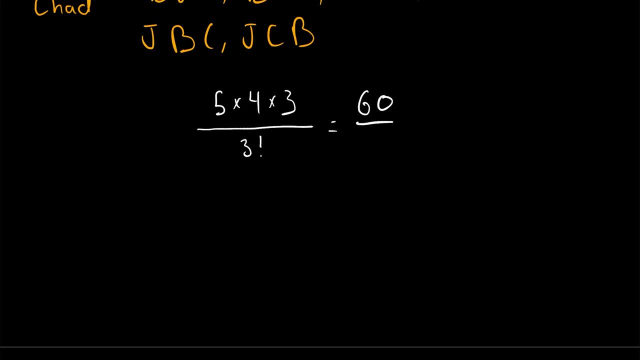 by three factorial, This will give us a final count of 60 divided by three factorial, which is six, and that's going to be equal to ten. That is the number of combinations of three objects from a collection of five, And you might say, okay, that looks kind of similar to the formula we saw at the beginning. 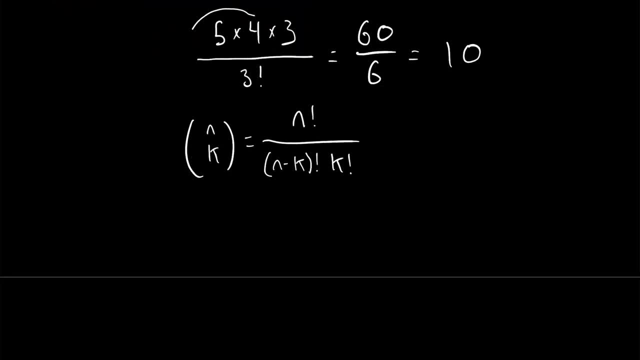 but it certainly doesn't look quite right. So how can we rewrite this in a form that looks more similar to the general formula? If we put five factorial in the numerator, so that we're trying to make something that looks more like this, then not only. 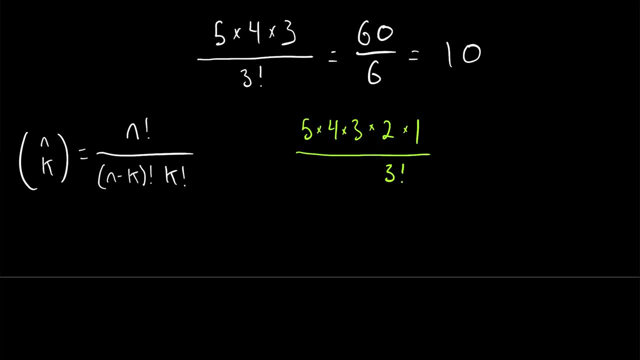 do we have to divide by three factorial, as we did before, to get rid of five factorial. but we also have to divide by three factorial, as we did before, to get rid of five factorial. So we have the alternate orderings of every combination of three actors, but we also have 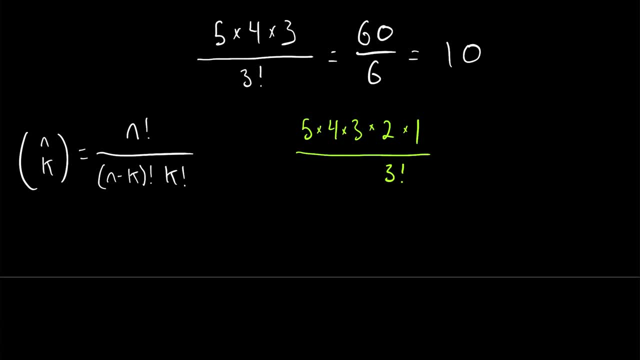 to divide out the number of orderings of actors that we're not selecting And since there are five actors and we are selecting three, the number of actors we aren't selecting is five minus three, So the number of ways of ordering those actors we're not selecting. 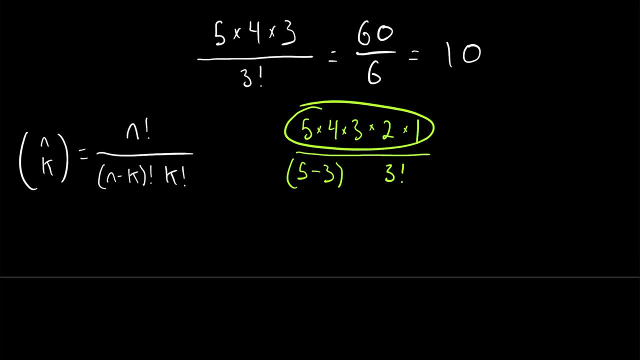 which are being counted here. we don't want them to be counted, which is why we're dividing them out. that number of ordering the actors we're not selecting is five minus three factorial, And now we see a form that resembles the formula. 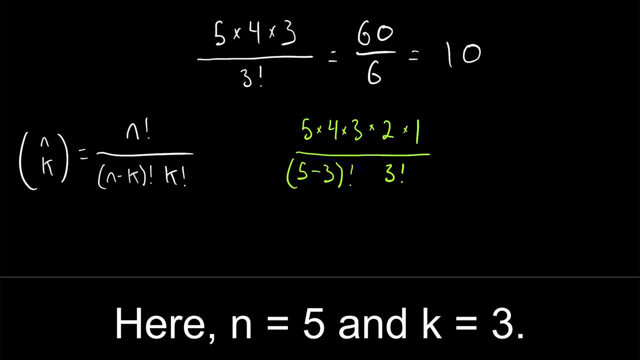 And that's a multiplication sign right there, but it looks kind of ugly. Let me just bring these numbers close together so we see they're getting multiplied. So this is the same thing we had above. We can see that pretty clearly, if I just 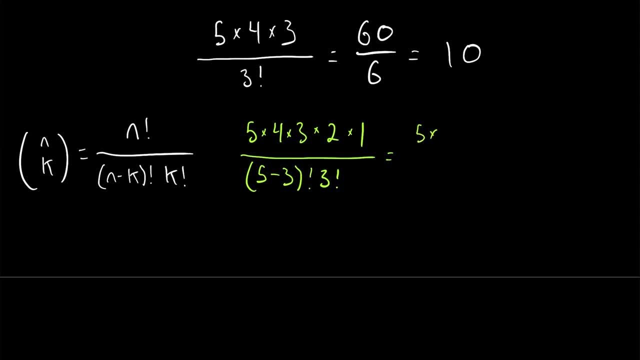 rewrite this a little bit. On the numerator we have that five factorial and then in the denominator we have five minus three factorial, which is two factorial, which is two times one, and then that's getting multiplied by three factorial And we see that two and one in the 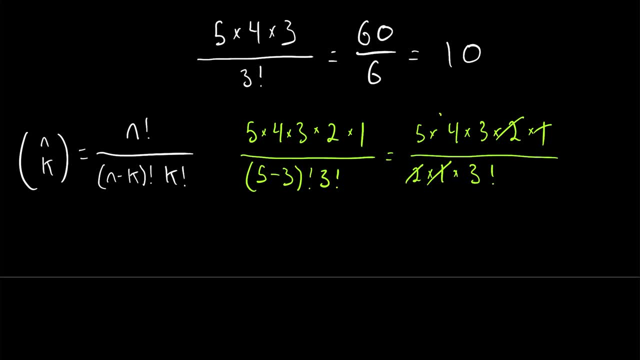 numerator and denominator cancel out and we're left with the same thing we had above, Five times four times three, divided by three factorial, And that is where the formula comes from. Again. this here is called a binomial coefficient. It's read n, choose k, It's the number. 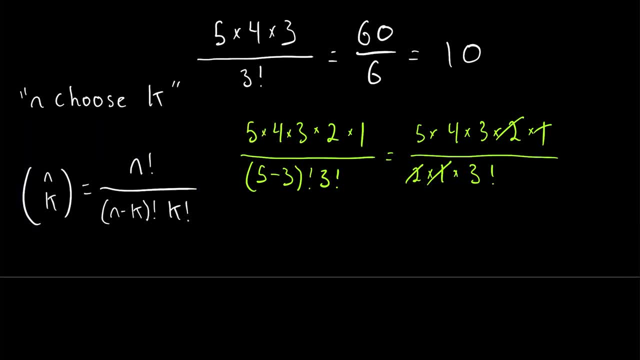 of ways we can choose k objects from a collection of n objects, where the order of selection doesn't matter. We're only interested in the combination of objects, which is why it's called the combination formula. The n factorial in the numerator is the number of ways of ordering. 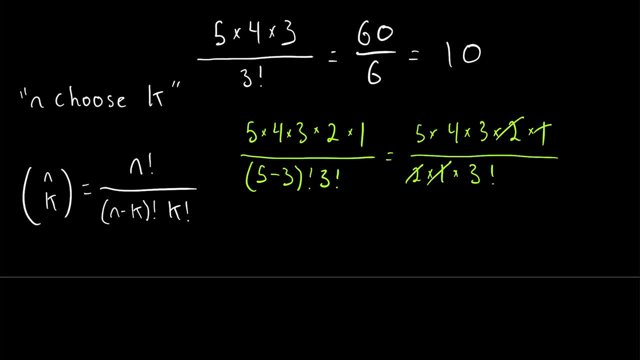 those n objects in the collection. But since we're only selecting k of them, there are n minus k objects that we are not selecting and there are n minus k factorial ways that those objects can be ordered. Since we're not selecting them, we don't care about their orderings. we divide that number.